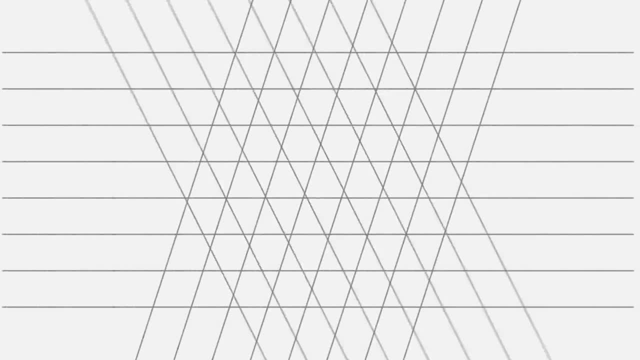 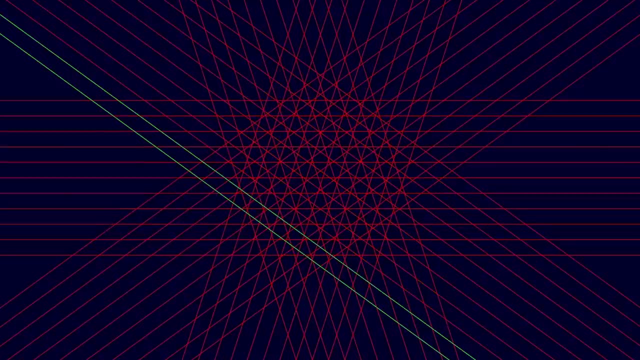 rotated and intersect at 60 degrees. And if you create a grid with five sets of lines evenly rotated from each other and intersecting at either 36 or 72 degrees, you get a pentagrid. Pentagrids are made up of five sets of parallel lines. 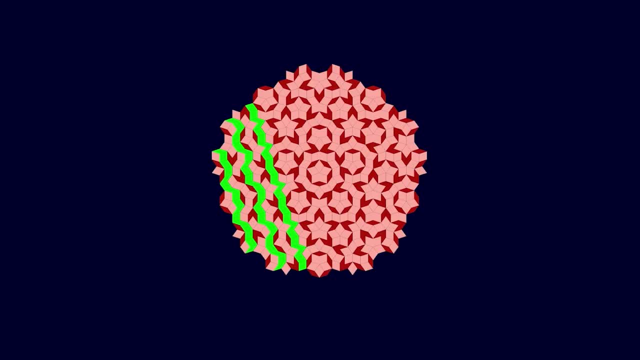 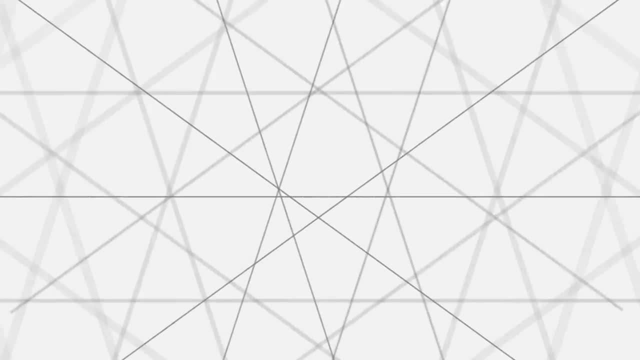 And Penrose tilings are made up of five sets of parallel ribbons of tiles, Because they're actually the same. To make a Penrose tiling, all you have to do is start with a pentagrid and then, at every point where two lines intersect, you draw a tile oriented, so the sides of the tiles. 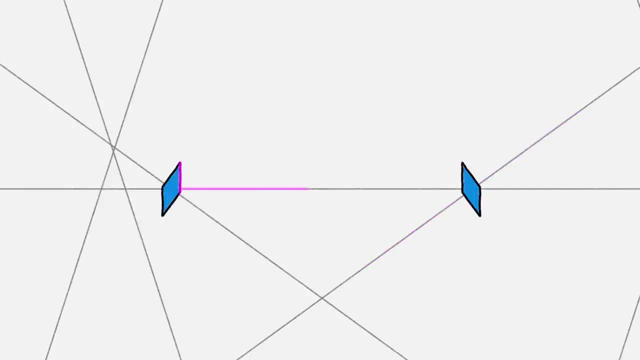 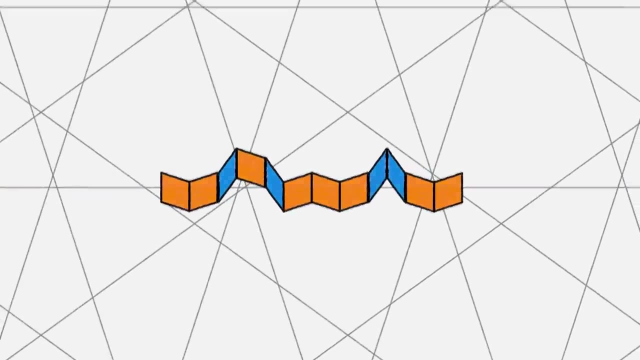 are perpendicular to the two lines. This way, at the next intersection along the line, the sides of that tile will be parallel to the sides of the first tile, and the same at the next intersection, and so on, and you can slide them all together into a ribbon And 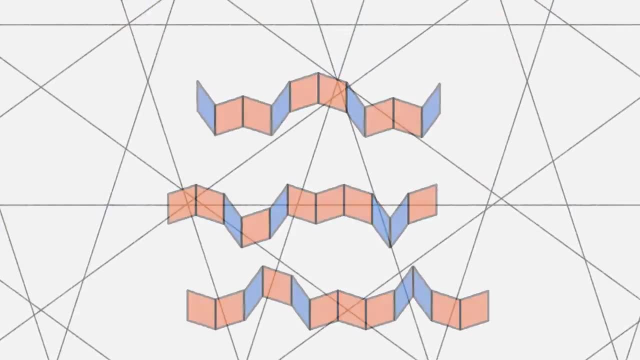 if you do the same for the next line up in the pentagrid, you get another ribbon and another. And if you also do it for all the other lines in the other directions, all the ribbons combined together make a Penrose tiling. 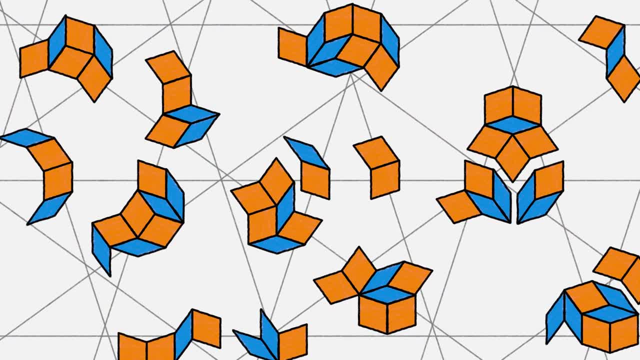 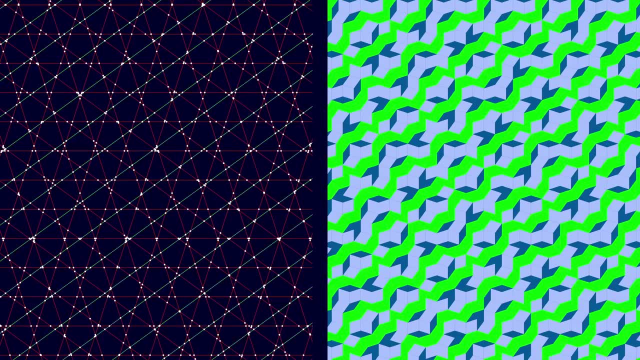 You can also just add a tile to every intersection and slide them all together along the grid lines. Either way, you get a Penrose tiling. Every Penrose tiling is made out of five infinite sets of parallel, infinitely long ribbons. 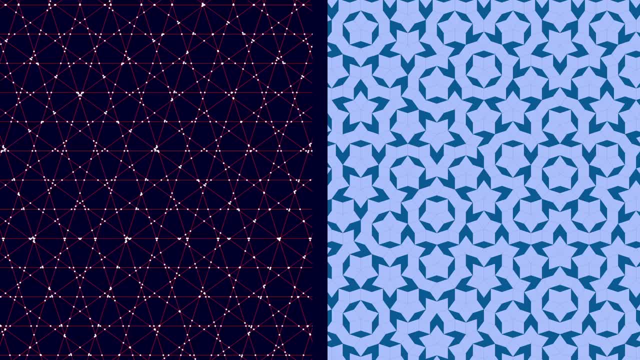 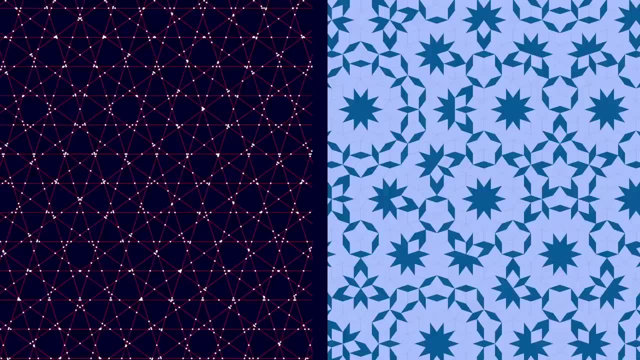 Because every Penrose tiling is a pentagrid in disguise. Of course, you don't have to use this particular pentagrid. We can also shift the various different sets of lines by random amounts And get a beautiful new tiling that's slightly different from Penrose tilings. 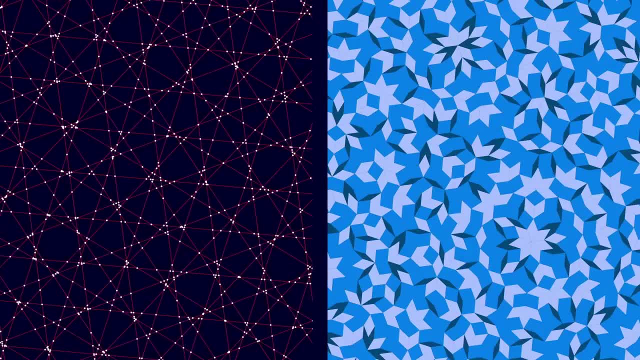 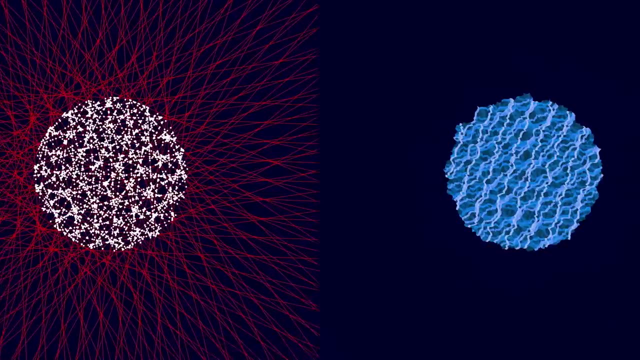 And we're not limited to a pentagrid. Here's a heptagrid and its corresponding Penrose-like tiling, And here's an octagrid, a nanagrid, a decagrid and so on. And that beautiful ribbony pattern we showed before was from a grid with 17 different sets. 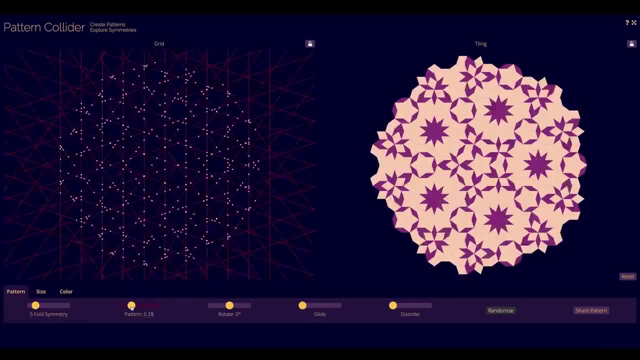 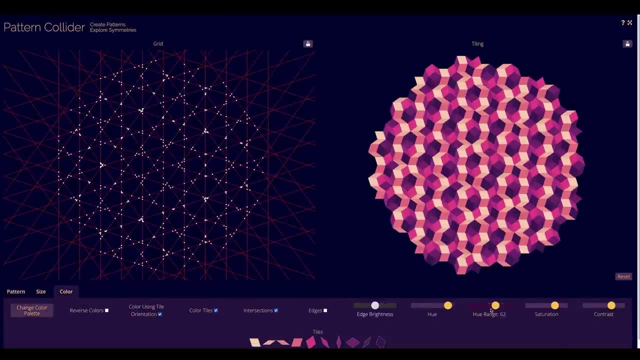 of lines. My friend Atish made an interactive website where you can play around with all of this and make your own Penrose-like patterns. You can highlight the grid lines and see their counterpart tiles and vice versa. You can change the colorings to bring out different. 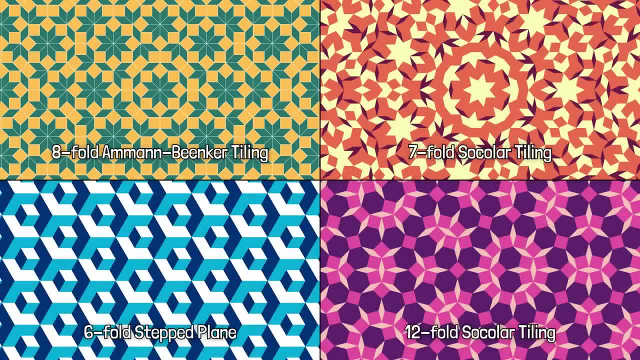 aspects of the patterns. You can use it to generate a bunch of other famous patterns. You can save them for a phone or computer background or to print on a shirt or whatever. It's really great and, as you've probably noticed, it's where all the visuals in this. 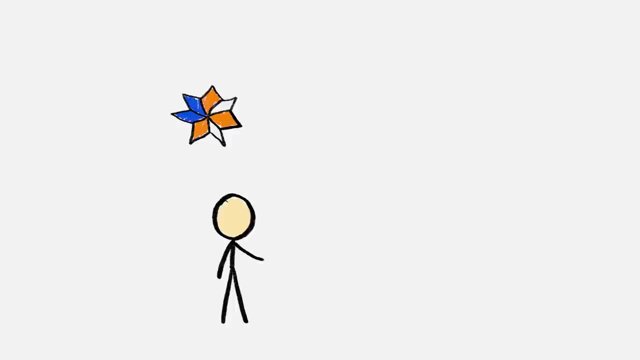 video are from. But there's one more thing. Remember how I said that pentagrids helped me see why these patterns never repeat themselves. This isn't a proof, but it at least gives you a flavor of the non-repetition. So start with a single ribbon. If the ribbon ever did repeat itself, then after a certain 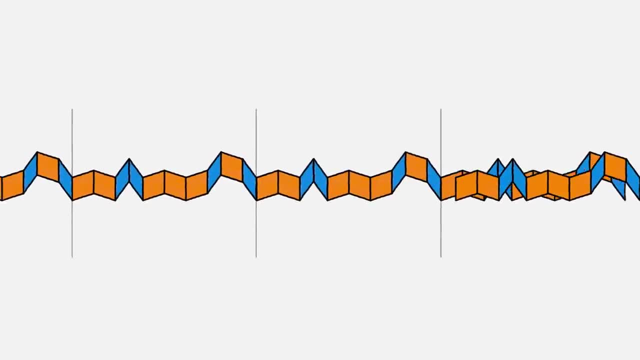 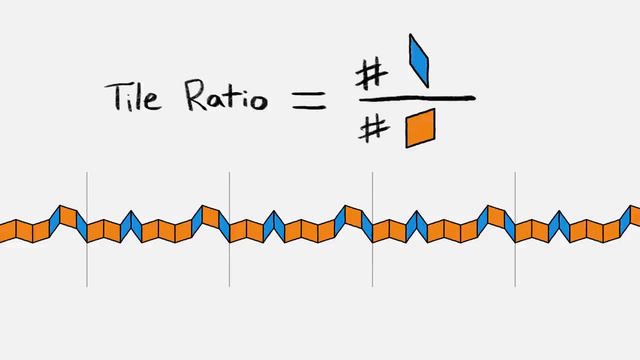 point in time you'd have the same pattern of thin and wide tiles over again And again And again. So the ratio of thin to wide tiles would be a rational number: The number of thin tiles in a given chunk divided by the number of wide tiles. In this example there. 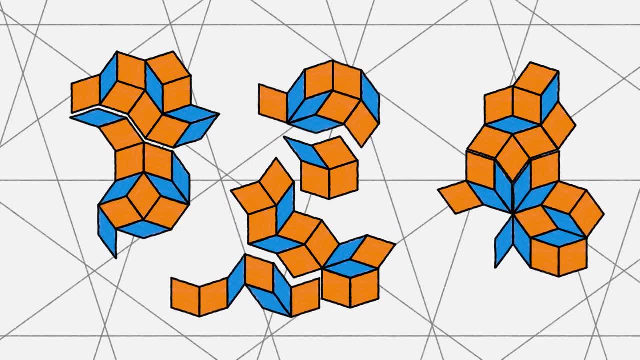 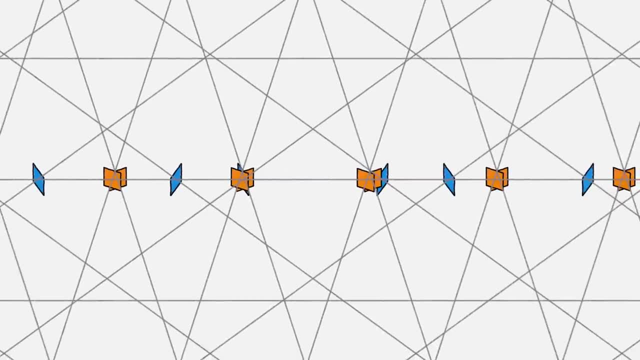 are six wide tiles for every four thin ones In an actual Penrose tiling. we can directly calculate the ratio of thin tiles to wide tiles, since the ribbons of tiles correspond to the intersections along a line of the pentagrid. The wide tiles are from the intersections. 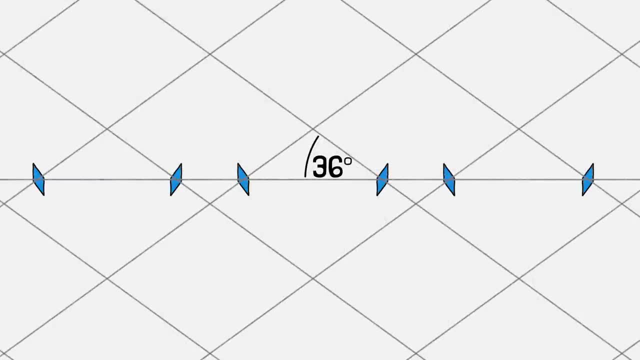 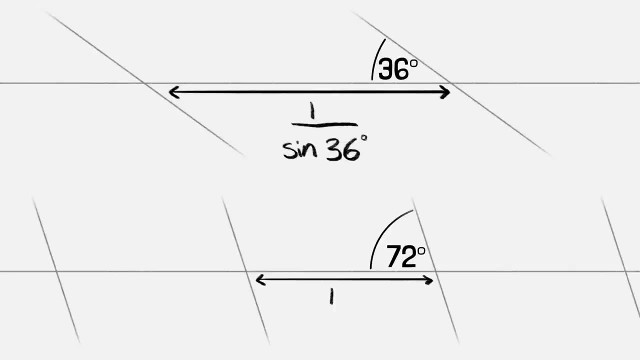 with the 72-degree lines and the thin tiles from the 36-degree lines. Some basic trigonometry shows that the spacing between 36-degree lines is 1 over the sine of 36 degrees and the spacing between 72-degree lines is 1 over the sine of 72 degrees. So 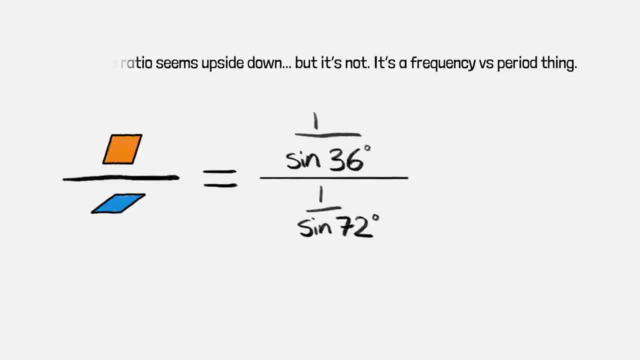 the ratio of wide tiles to thin tiles is the ratio of these, which happens to be the golden ratio, which is irrational. So there's no way the pattern could ever repeat. If it did, the golden ratio would have to be rational. Remember, if the pattern did repeat the ratio. 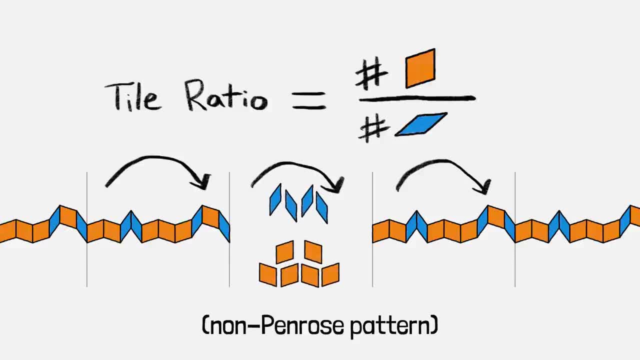 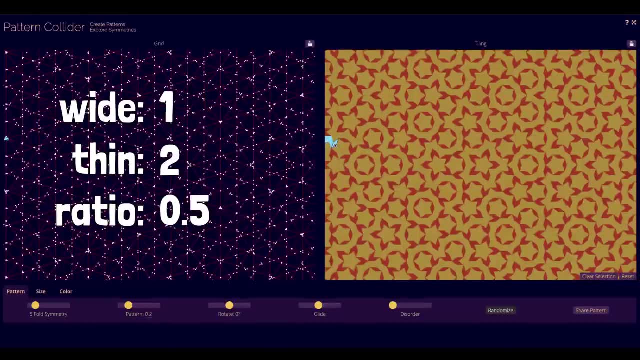 of wide to thin tiles would have to be rational, which the golden ratio isn't, Of course. this just proves the tiling can't repeat in one direction. The whole proof is a little bit more than we want to get into here. The pentagrid allows us to directly calculate. 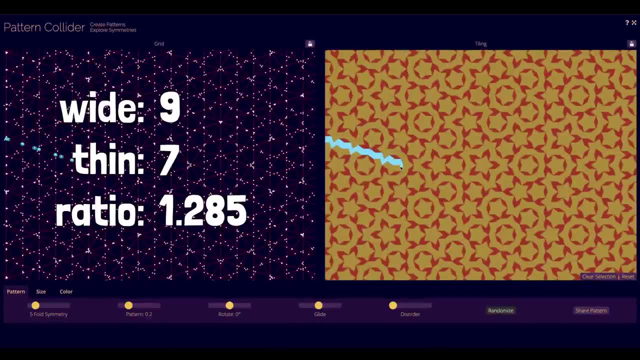 that as you go out along any ribbon, in a Penrose tiling for every 10 thin tiles you see there are on average 16.18 wide tiles, a golden ratio worth. And because the golden ratio is irrational, sometimes there are slightly more wide tiles for every 10 thin ones. and 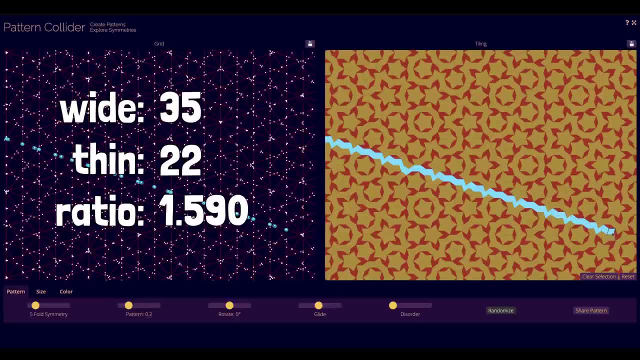 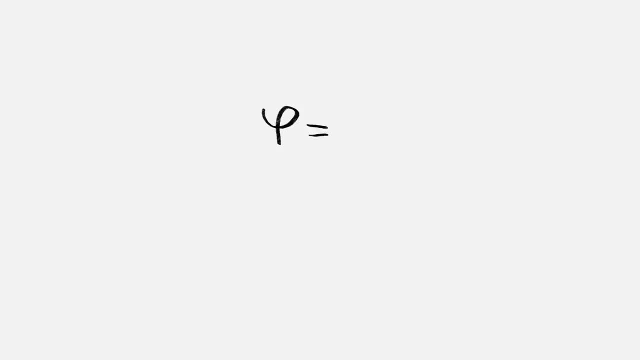 sometimes there are slightly fewer, in a way that is perfectly predicted by the value of the golden ratio, but never repeats, And the more tiles you look at, the more closely their ratio matches the golden ratio. Of course there's nothing special about the golden. 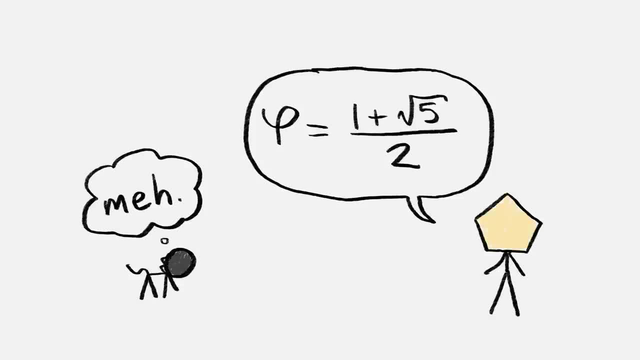 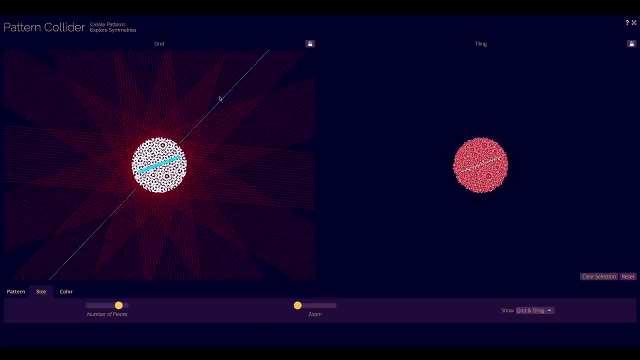 ratio here. It happens to show up a lot when you have five-sided things For the heptagrid or decagrid or whatever. the ribbons still don't repeat because the ratio of the space spacings with the grids and the ratios of the numbers of types of tiles is some other. 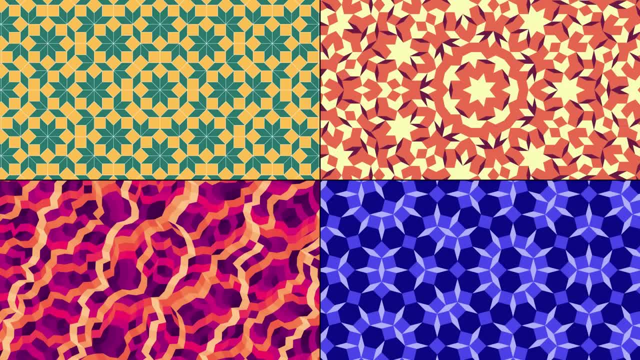 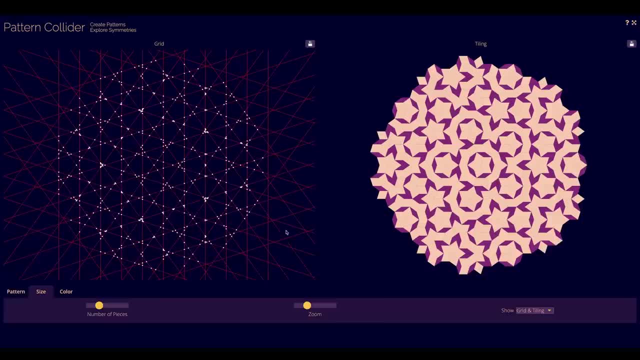 irrational number. All these patterns are quasi-periodic. They may never repeat. but they also aren't just a random jumble of tiles. All right, go play with the beautiful Penrose tile patterns over at atishbcom: slash patterncollider.